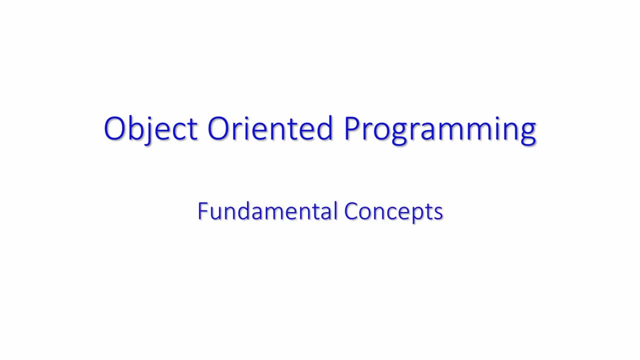 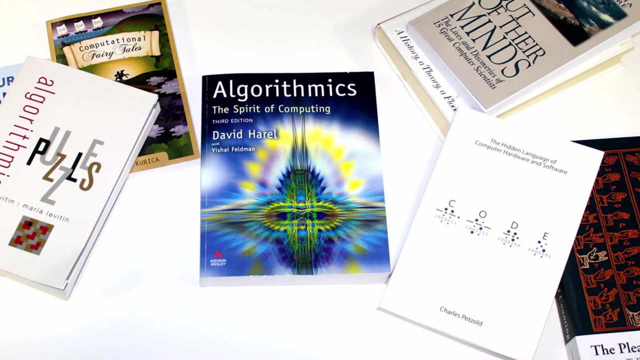 The four fundamental concepts of Object Oriented Programming are Abstraction, Encapsulation, Inheritance and Polymorphism. Before considering what they mean, first consider what is an object. An object is a thing from the real world. It could be a car, a boat or a book. 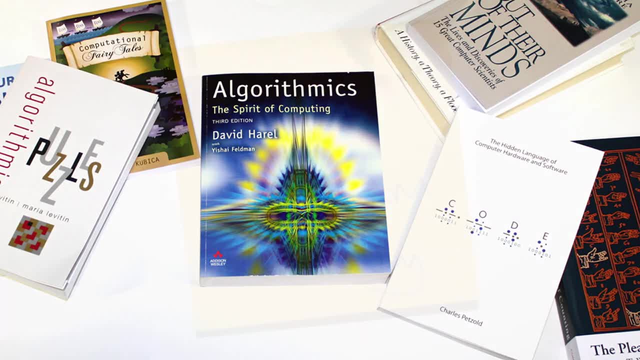 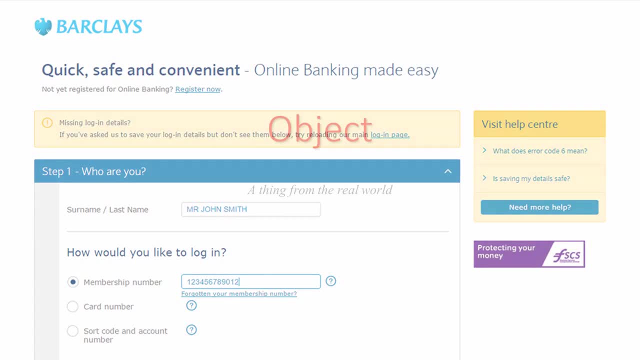 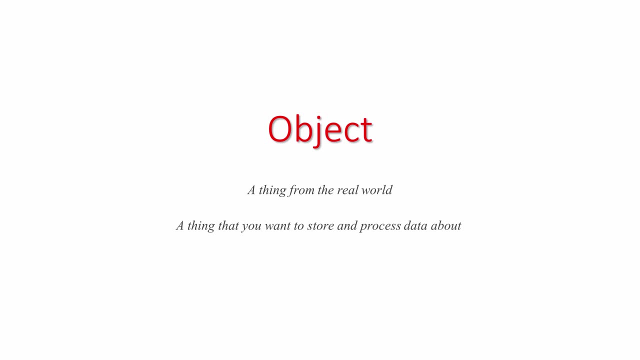 But it might not be something physical that you can touch. It could be a dental appointment, a seat reservation for the cinema or a bank account. In the realm of Object Oriented Programming, an object is anything of interest to the software application that you're building. It's. 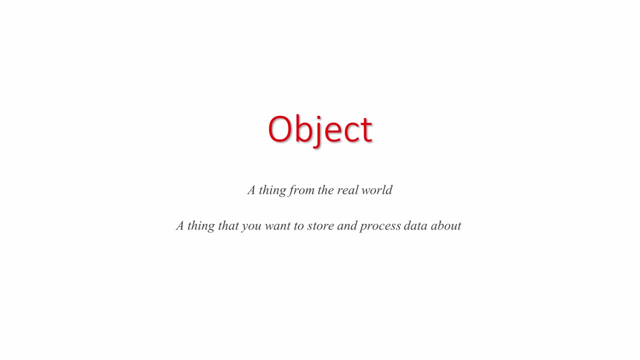 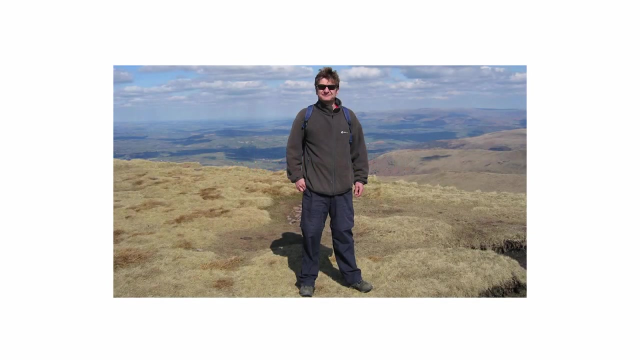 anything that you want to store and process data about. Another name for an object is an entity. This leads us to the first fundamental concept of Object Oriented Programming, namely Abstraction. Abstraction means to simplify reality. For example, a person is an object, But if you were designing a new application, you could. 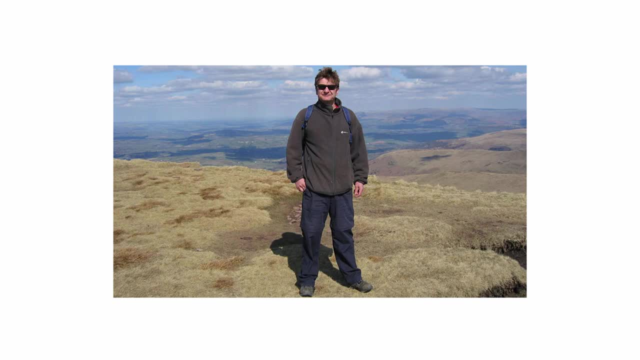 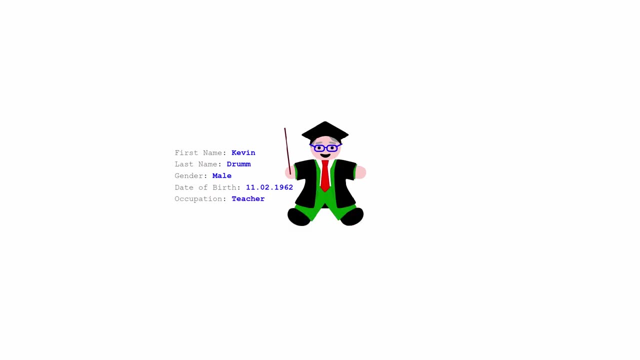 use an entity to process data about a person, It's unlikely that you'd be interested in everything there is to know about a person. Rather, you would only concern yourself with the data that are relevant and the tasks that you want to perform with those data. 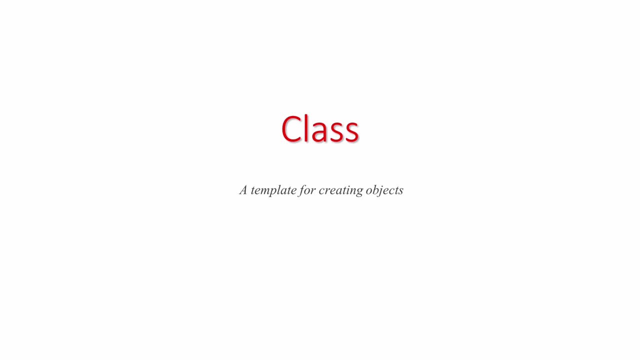 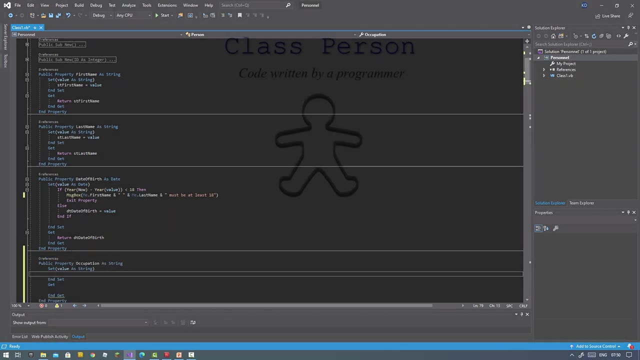 To create objects programmatically, you need a class. A class is a template for creating objects. A class is code written by a programmer to define the attributes and the objects. A class is a group of variables that represent the properties of an object. Attributes describe: 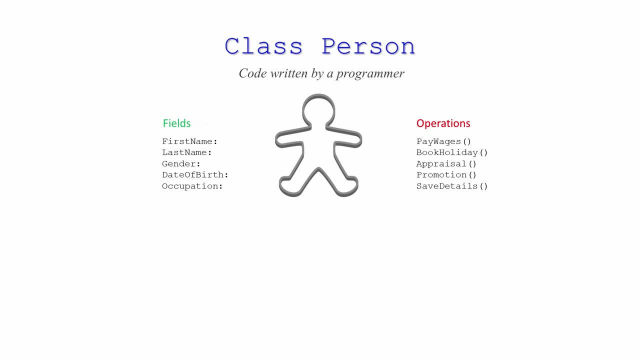 the object. They're sometimes referred to as fields, because they contain data. Most programmers know them as properties. Properties are coded within the class either as public variables or as property procedures. Operations are actions that can be done to or performed by the object. They're sometimes referred to as behaviours, but more commonly they're 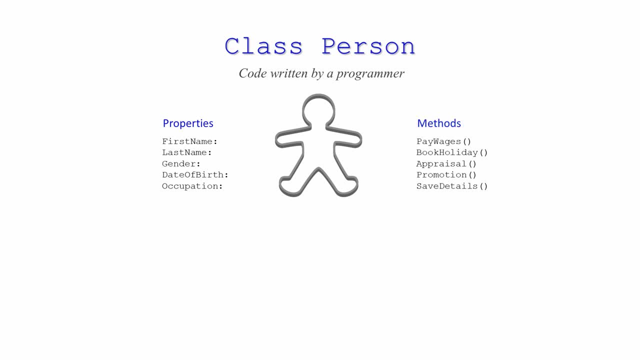 known as methods. Methods are programmed to produce a specific result using data. When you create an object, a specific result that is asked of you will be determined by the properties and the actions programs within the class that are coded either as procedures or functions. 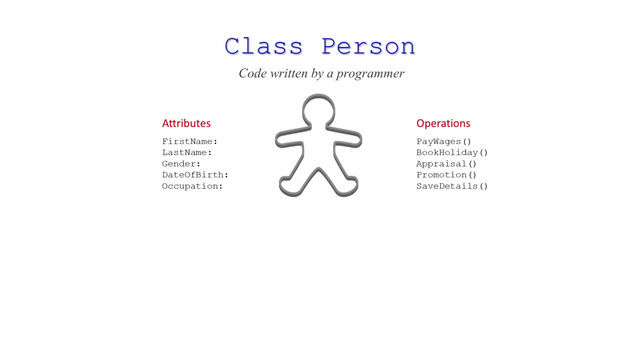 operations of an object. Attributes describe the object. They're sometimes referred to as fields because they contain data. Most programmers know them as properties. Properties are coded within the class, either as public variables or as property procedures. Operations are actions that can be done to or performed by the object. They're sometimes referred 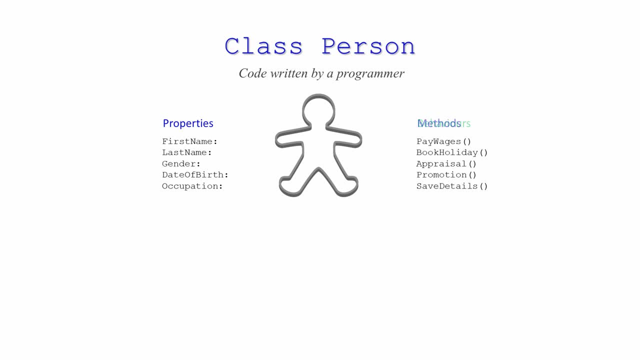 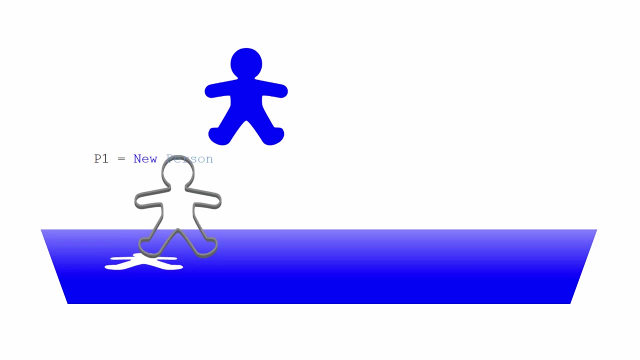 to as behaviours, but more commonly they're known as methods. Methods are processes that are programmed within the class, that are coded either as procedures or functions. A class is a template for creating objects, and it's often compared with a pastry cutter, because once it's been written, it can be used to create many objects of the same type. 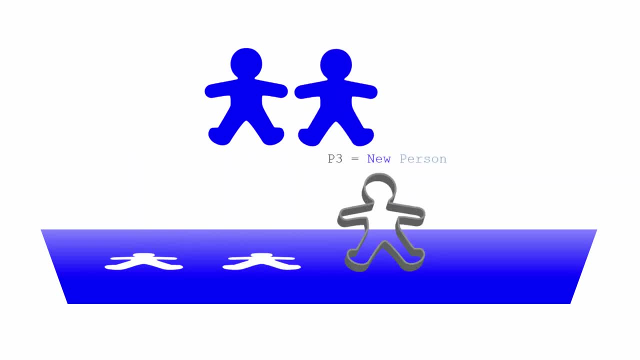 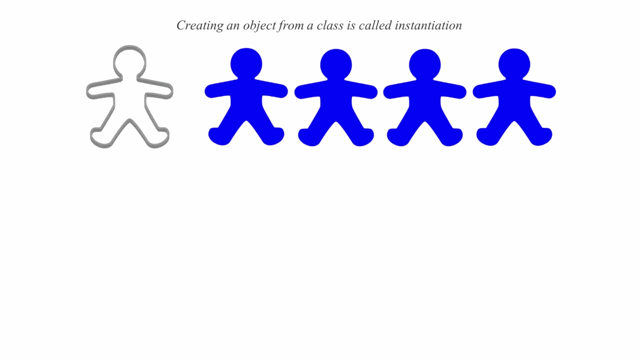 In fact, a class is sometimes referred to as a type. Each object is an instance of a class in the computer's memory. Creating an object from a class is therefore known as instantiation. Once these objects have been created, their properties can be assigned values, making each object of the 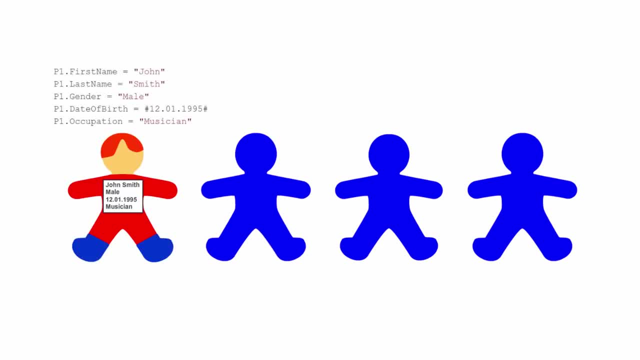 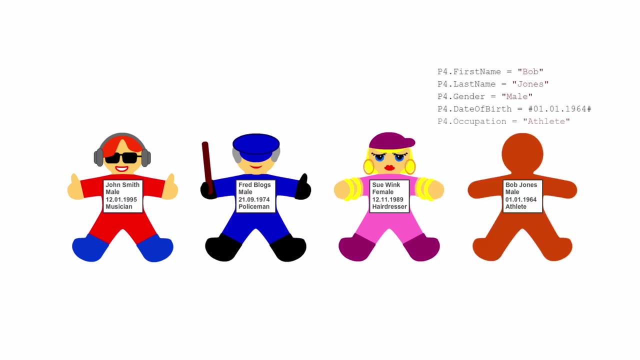 same type, a unique entity. Each property is defined in the class by a property procedure, which may include code to validate a property value while it's being assigned. This helps to ensure the integrity of the data contained within the object. The property values that have been assigned to an object are collectively known as the. 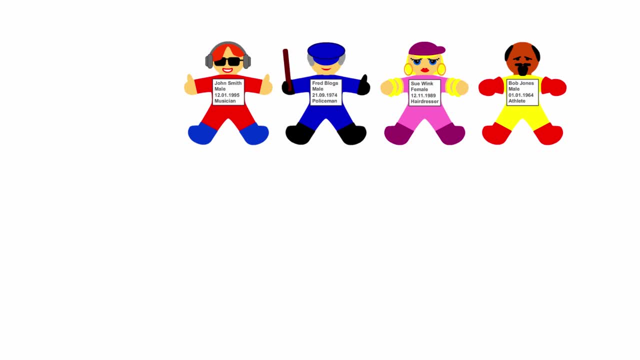 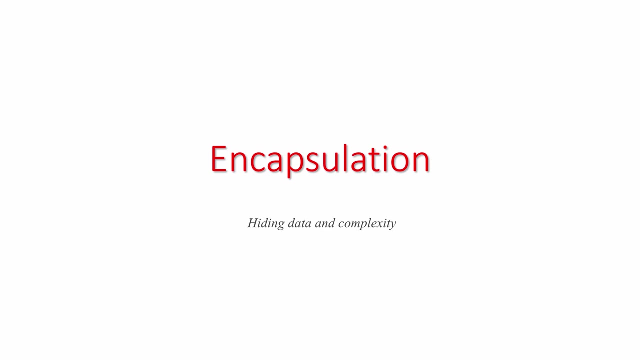 state of the object. It's also possible to assign values to properties, while an object is being instantiated by means of a special method called new. This method is known as the constructor. The second fundamental concept of object-oriented programming is encapsulation. This means to hide the complexity of the inner workings of an object from the programs. 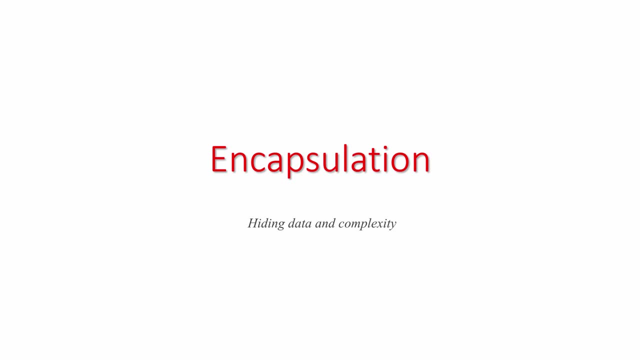 and the programmers that make use of it. It's often referred to as information hiding, because the data contained within an object and the functions that manipulate the data are bound together and therefore safe from outside interference. In some big software development projects, it's common for more experienced programmers. 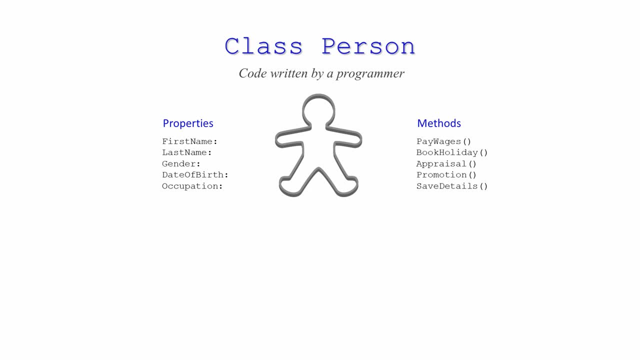 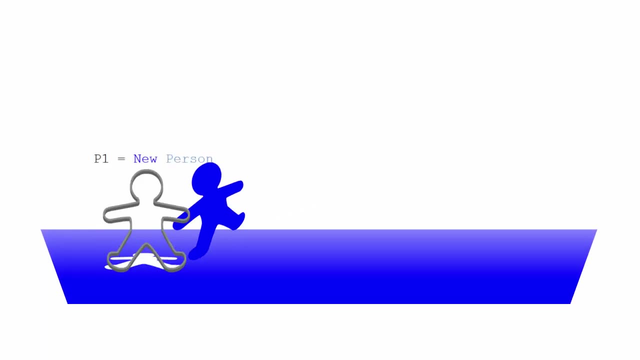 A class is a template for creating objects, and it's often compared with a pastry cutter, because once it's been written, it can be used to create many objects of the same type. In fact, a class is sometimes referred to as a type. 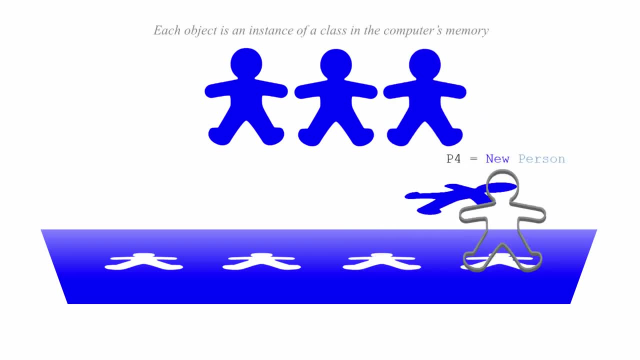 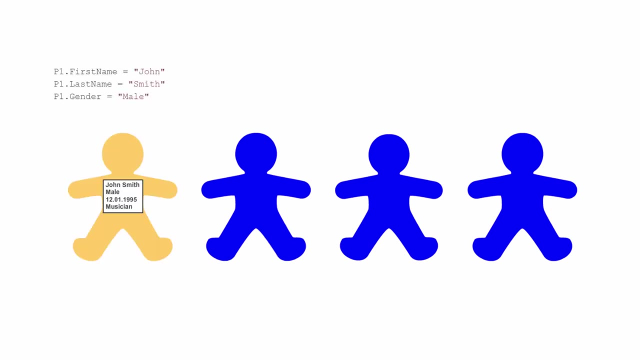 Each object is an instance of a class in the computer's memory. Creating an object from a class is therefore known as instantiation. Once these objects have been created, their properties can be assigned values, making each object of the same type a unique entity. 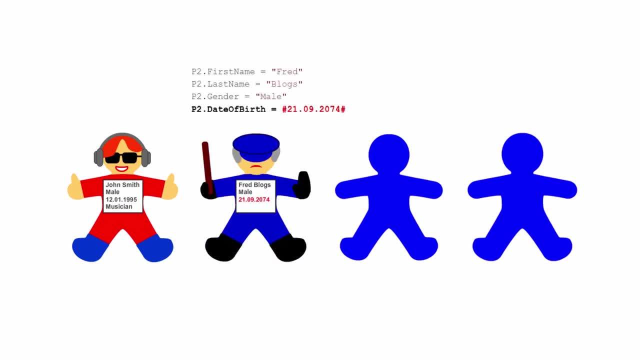 Each property is defined in the class by a property procedure, which may include code to validate a property value while it's being assigned. This helps to ensure the integrity of the data contained within the object. The property values that have been assigned to an object are collectively known as the. 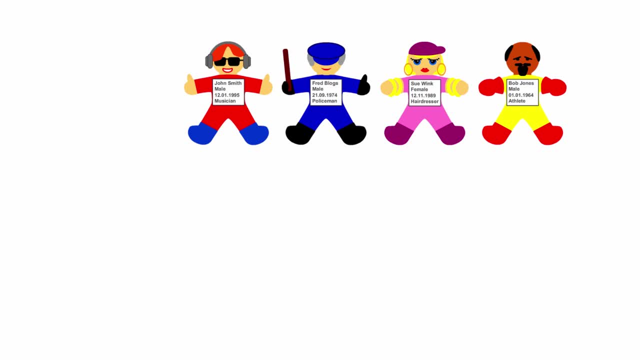 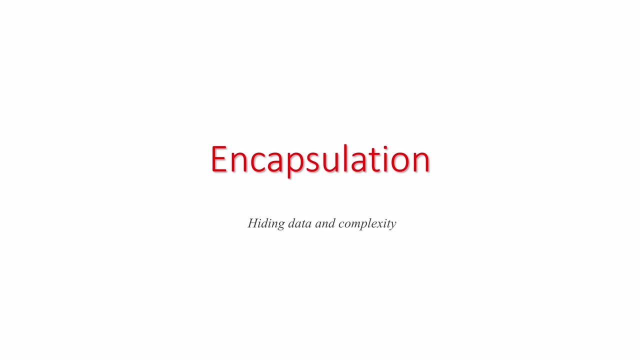 state of the object. It's also possible to assign values to properties, while an object is being instantiated by means of a special method called new. This method is known as the constructor. The second fundamental concept of object-oriented programming is encapsulation. This means to hide the complexity of the inner workings of an object from the programs and 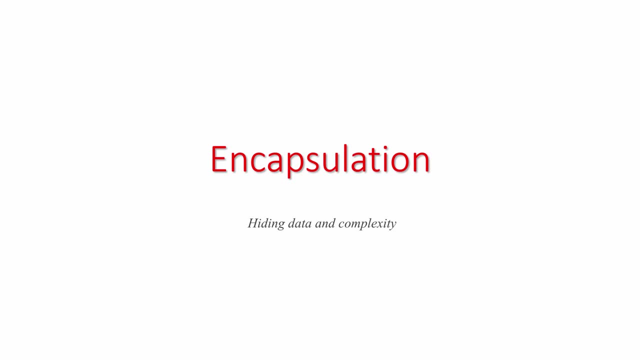 the programmers that make use of it. It's often referred to as information hiding, because the data contained within an object and the functions that manipulate the data are bound together and therefore safe from outside interference. The second fundamental concept of object-oriented programming is encapsulation. 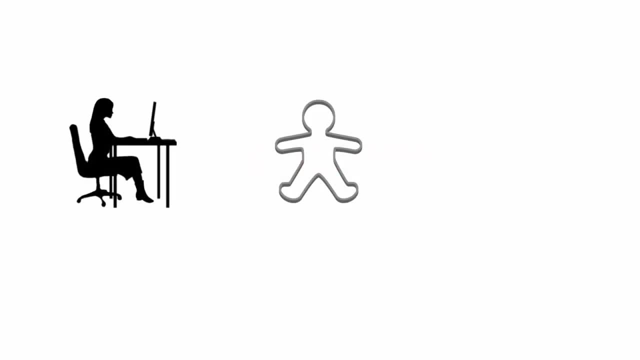 In some big software development projects, it's common for more experienced programmers to write the classes that will be used by the junior programmers. A class might be made available in the form of a class library. Indeed, some software development companies specialize in developing new classes to be. 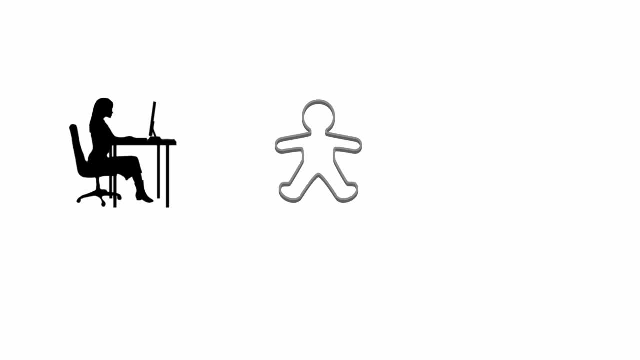 to write the classes that will be used by the junior programmers. A class might be made available in the form of a class library. Indeed, some software development companies specialise in developing new classes to be used by other software developers. Compiled class libraries protect their intellectual property. To write code that will create an 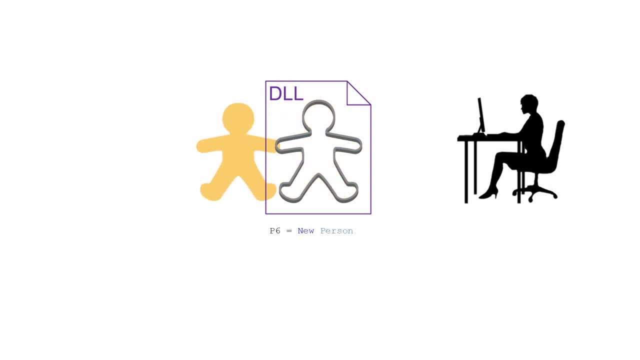 object from a class, then set its properties to a class. library is a common practice in software development. However, as software development is a complex process, it is often also difficult to understand the inner workings of the class. All a programmer needs to know is the name of the class, the properties and methods available. 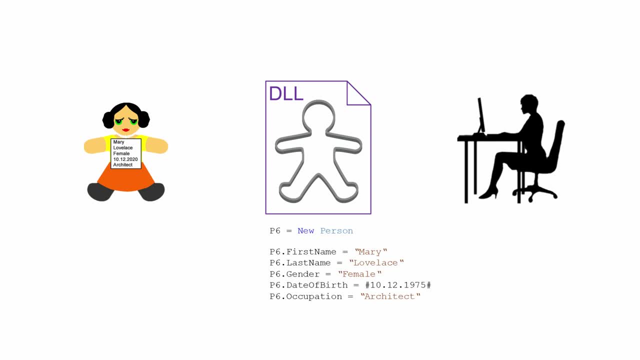 and any data that needs to be supplied when they are called. In other words, all our programmer really needs to know about is the interface of the class. The implementation code of those properties and methods can remain a mystery. This greatly simplifies the use of objects that can be used to create objects. 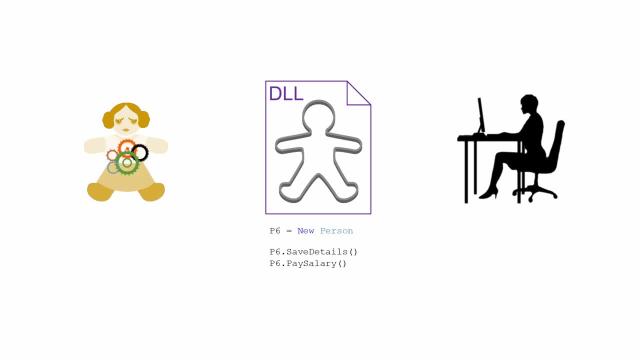 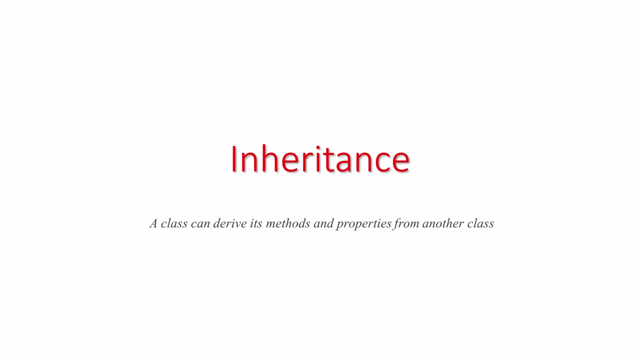 Let's take a look at some of the methods we use to create objects and helps to ensure that the data and operations encapsulated within are safe. The third fundamental concept of object-oriented programming is inheritance. This means that a class can derive its methods and properties from another class. 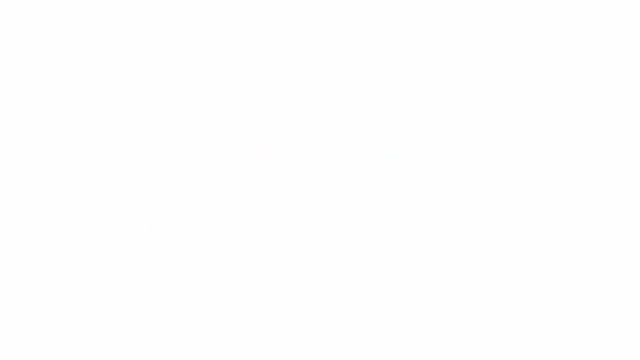 Inheritance can result in a hierarchy of classes. For example, this person class defines the methods and properties of a person. object: An employee in a business is also a person. so through inheritance, an employee class derives the methods and properties of the person class. 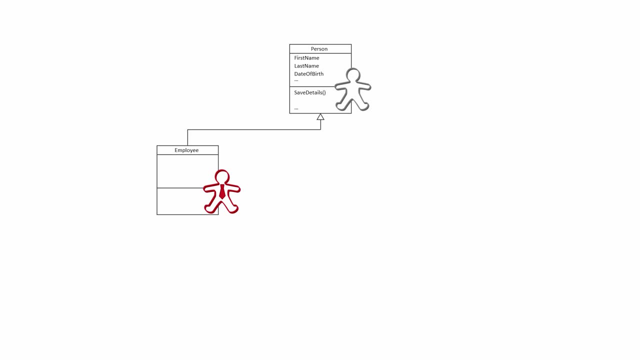 An employee is a type of person. A customer of the business is also a person. so through inheritance a customer class also derives the methods and properties of the person class methods and properties of the person class. A customer is a type of person- An employee. 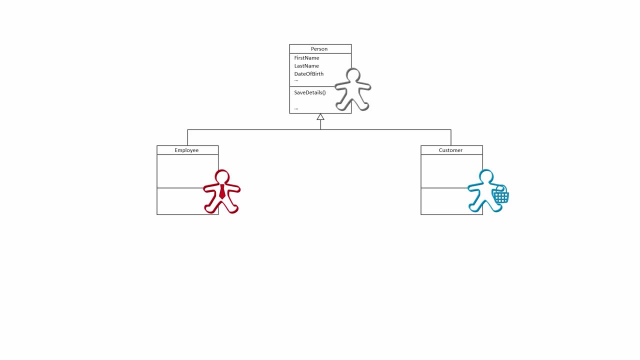 class can have some extra properties and methods of its own. It can extend the person class And so can a customer, But it need not stop there. A programmer is a type of employee, And so is a manager, and a cleaner Inheritance defines type of. 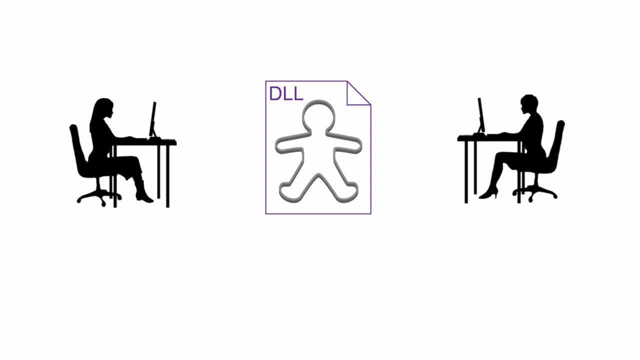 used by other software developers. Compiled class libraries protect their intellectual property. To write code that will create an object from a class, then set its properties and call its methods. it's not necessary to understand the inner workings of the class. All a programmer needs to know is the name of the class, the properties and methods available. 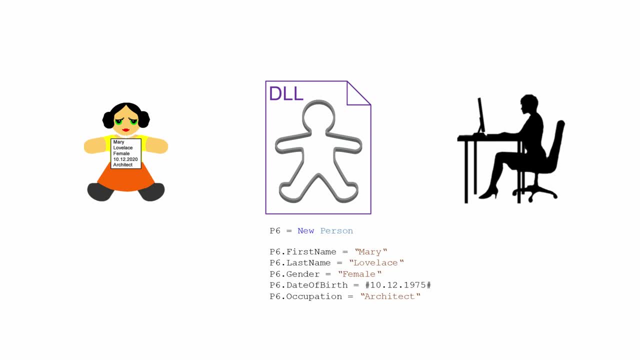 and any data that need to be supplied when they're called. In other words, all our programmer really needs to know about is the interface of the class. The documentation code of those properties and methods can remain a mystery. This greatly simplifies the use of objects and helps to ensure that the data and operations 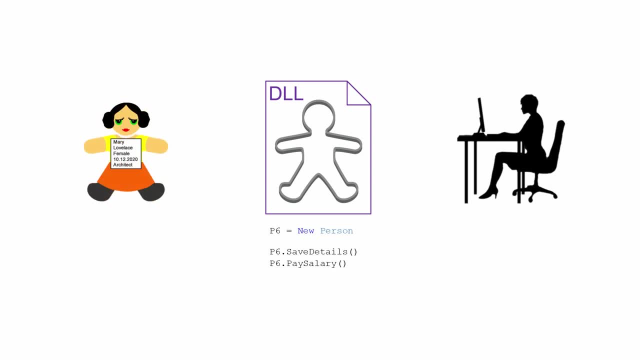 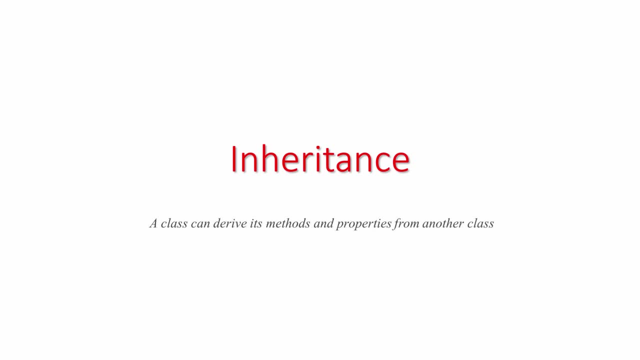 encapsulated within are safe. The third fundamental concept of object-oriented programming is inheritance. This means that a class can derive its methods and properties from another class. For example, this person class defines the methods and properties of a person object. 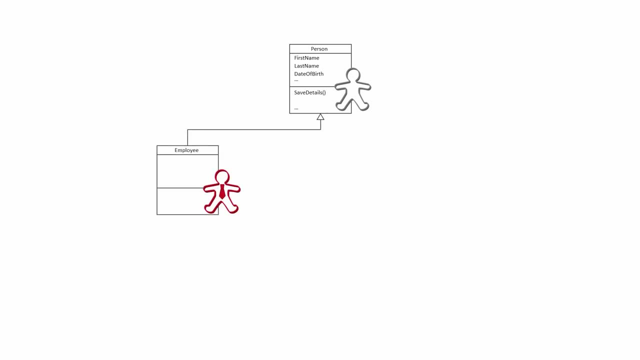 An employee in a business is also a person, so through inheritance, an employee class derives the methods and properties of the person. class An employee is a type of person. A customer of the business is also a person, so through inheritance, a customer class is. 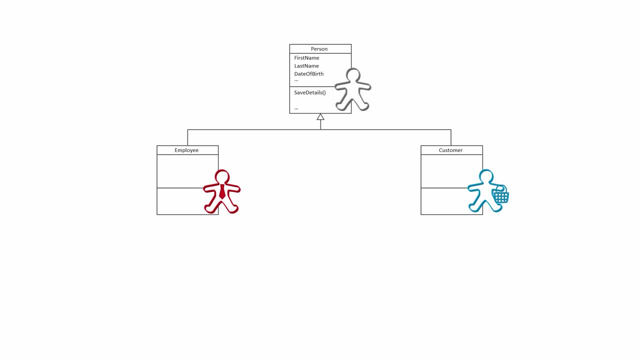 also a person. A customer class also derives the methods and properties of the person class. A customer is a type of person. An employee class can have some extra properties and methods of its own. It can extend the person class And so can a customer. 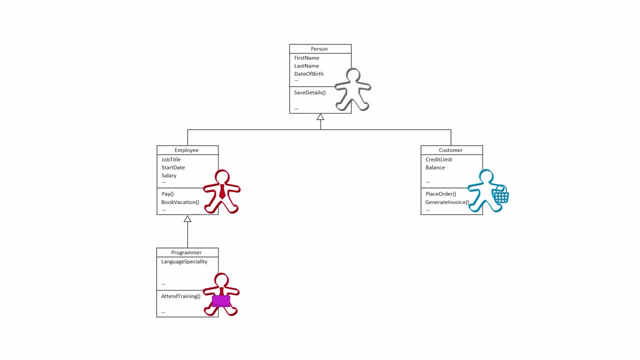 But it need not stop there. A programmer is a type of employee, And so is a manager and a cleaner. Inheritance defines TYPE OF relationships. The class at the start of inheritance hierarchy is called the BASE class. Any class that derives from another class is called A SUBCLASS.